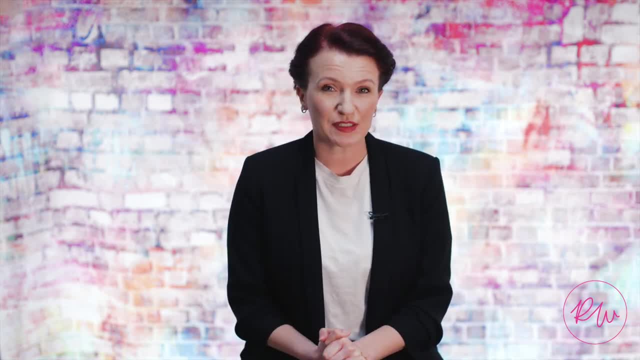 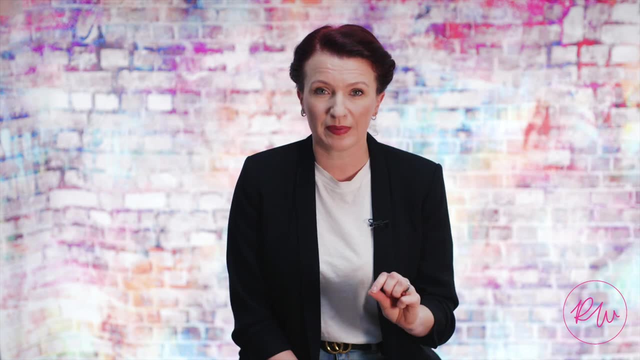 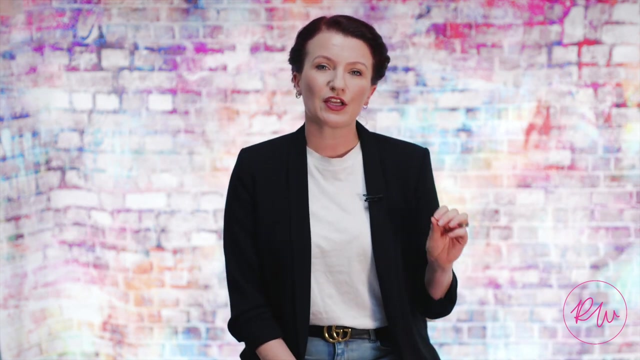 Hello and welcome back to my channel. In today's video, I'm going to give you five really great tips if you are at the start of your public speaking journey. So if you're very new to speaking in public, or if you're somebody who is nervous about speaking in public, these tips are for you. 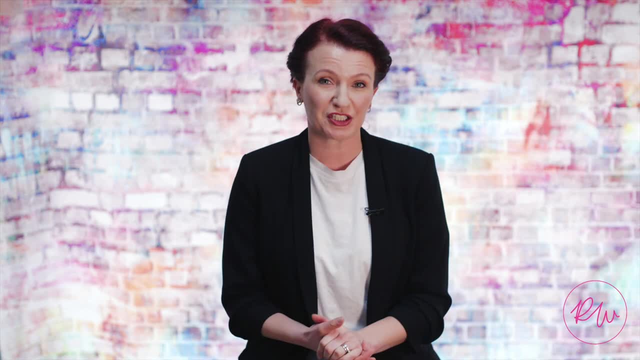 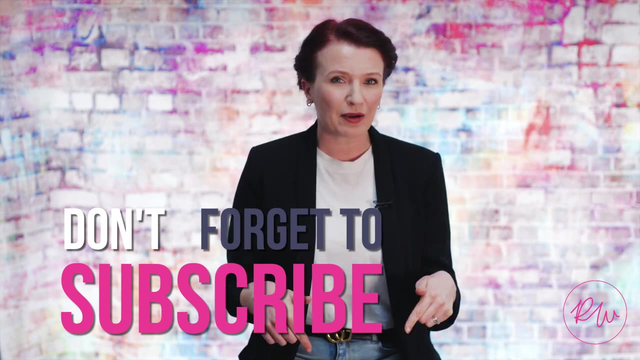 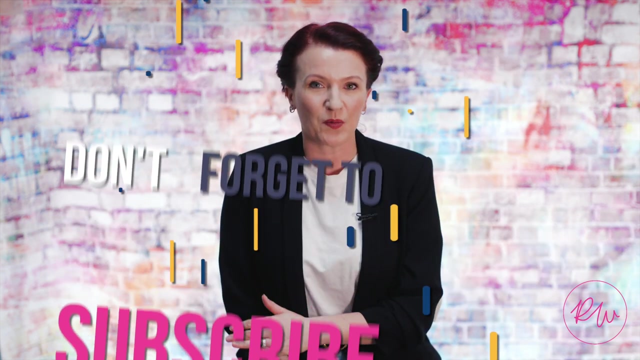 As always, please do subscribe to my channel. I often get asked if I do any one-to-one speaker coaching, and I do. Any details about me are on my website and you can check out that information in the description bar below. Let's get on with this video. 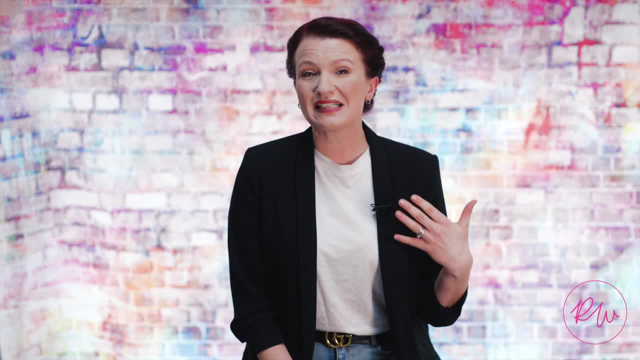 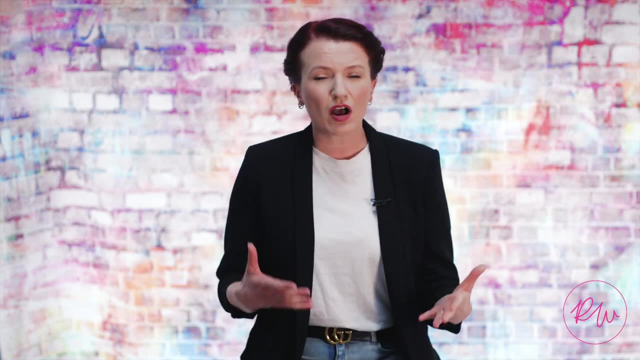 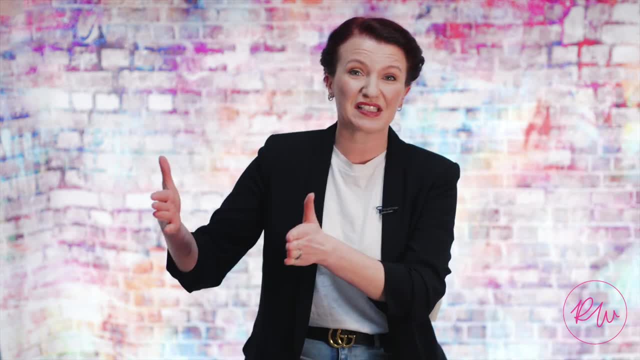 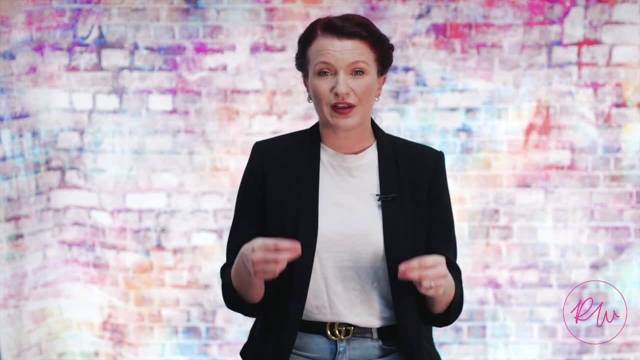 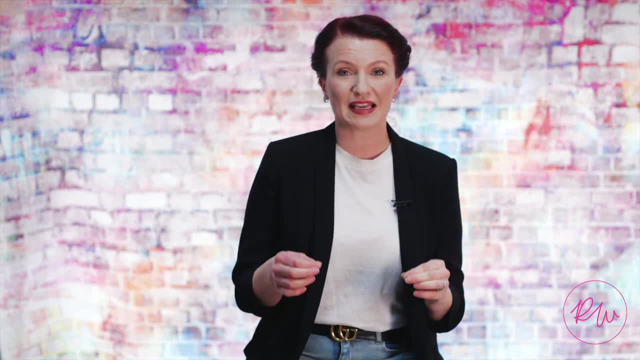 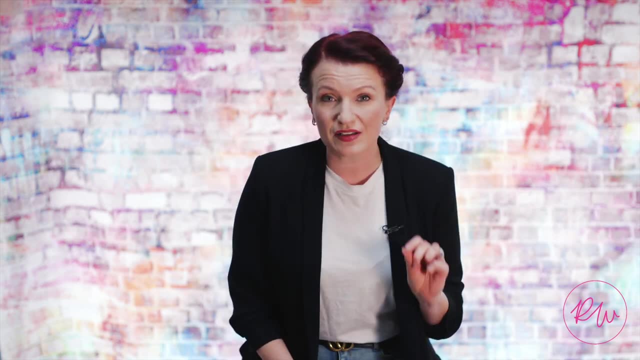 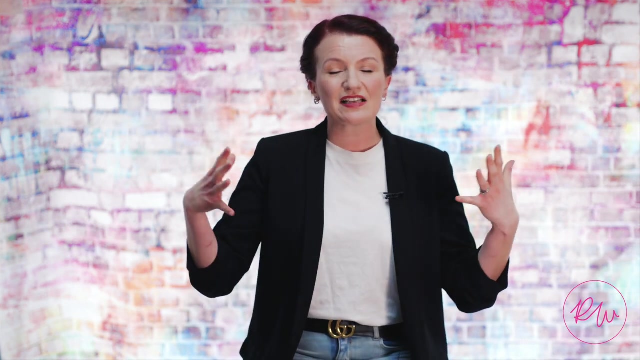 important one, and that is keep it simple. One of my favorite phrases is: keep it simple and do it well. Now, that does not mean dumbing down your content if what you're talking about is very complex, but it means instead of trying to boil the ocean and including everything in a presentation. 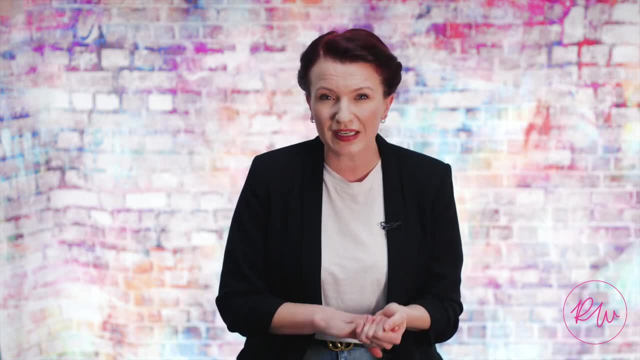 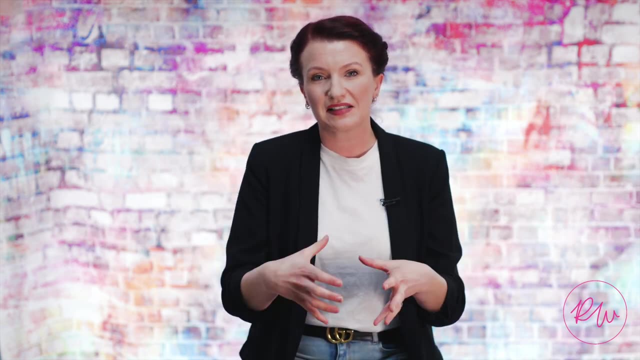 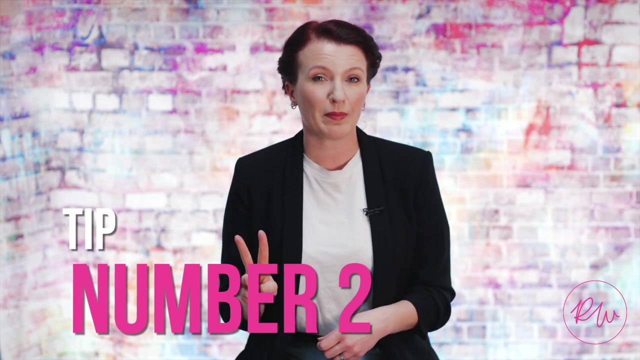 make sure you remember that the audience can only really take away three key messages. So you want to condense down? Always condense down your content. That is what I mean by keep it simple. Tip number two: Tip number two is all about control. If you're new to public speaking or if you're very nervous. 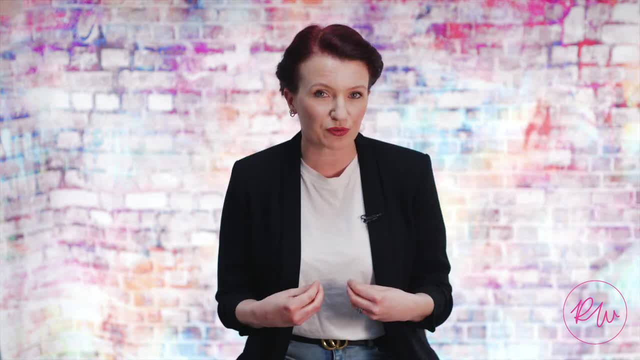 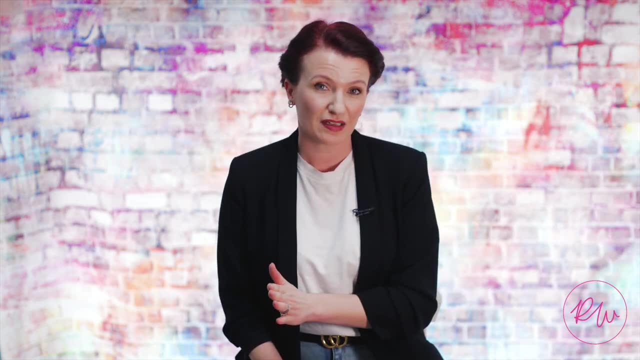 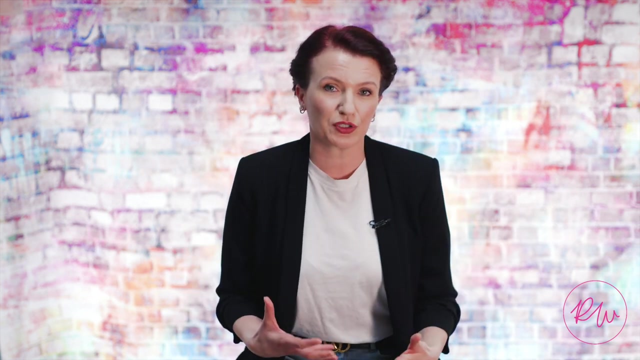 you need to learn how to control your instrument, and that is your voice. The main thing that most presenters get wrong is the speed at which they deliver their presentation. When you are under pressure, when you feel the adrenaline rushing through your body, your heart is beating faster. 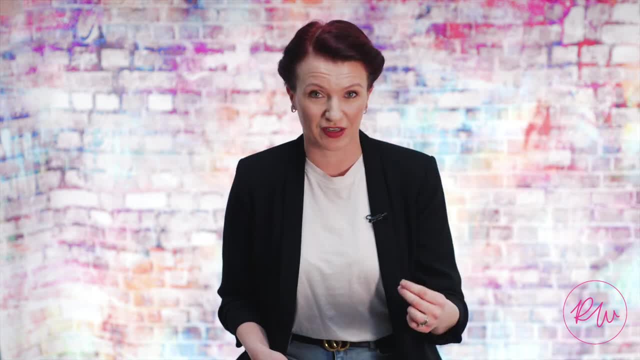 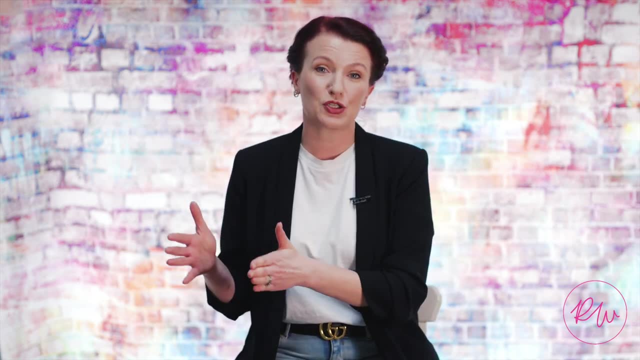 and a lot of the time you start to speak faster. So if you're new to public speaking or if you're really nervous, you need to learn how to control your instrument. The problem with speaking faster is the faster you speak, the harder it is to breathe, and that is where you can get into some really. 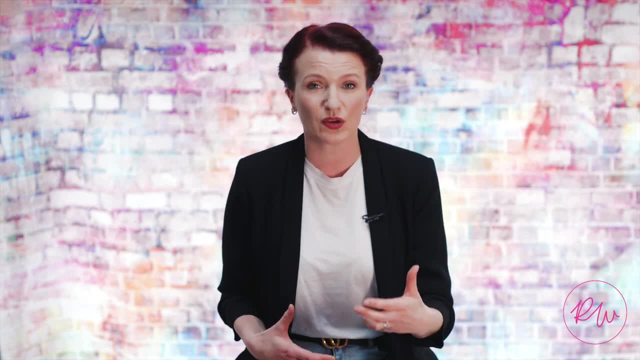 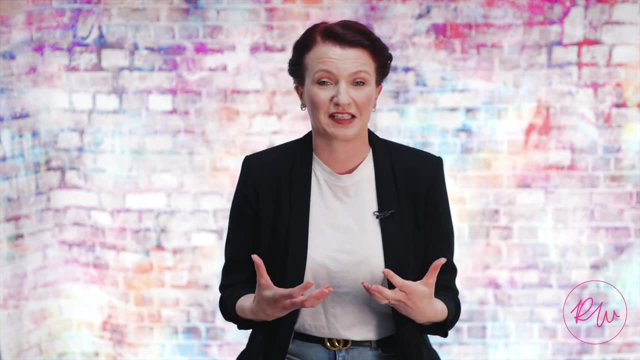 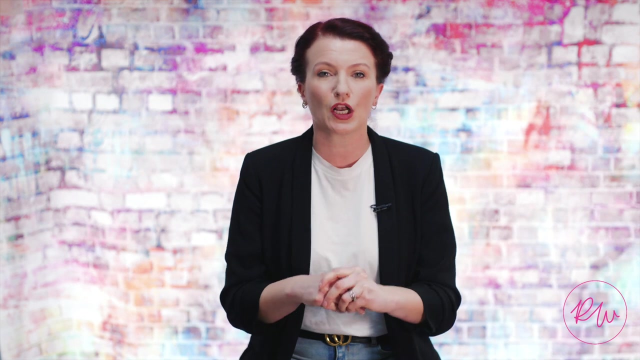 sticky situations on stage or in front of any audience where you're trying to catch your breath, The whole focus goes on to the fact that you're struggling to breathe and you lose concentration of where you are in your presentation. It's a horrible feeling that's pretty closely aligned to. 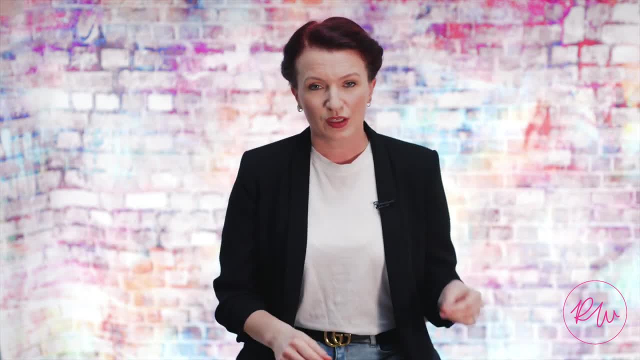 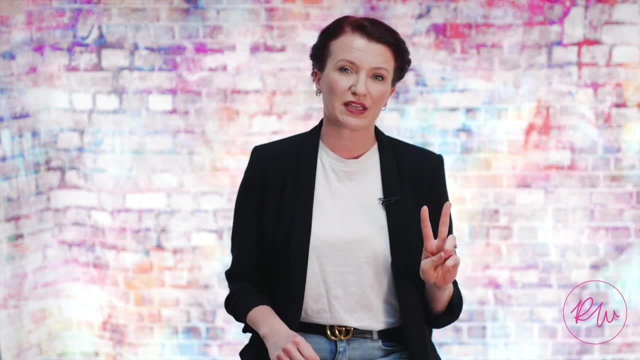 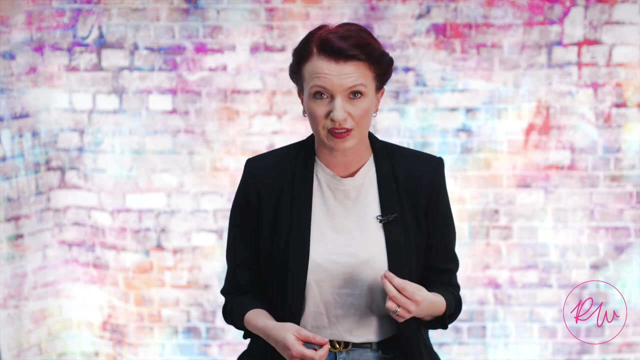 stage fright, So you don't want to go anywhere near that. You need to learn how to control your breathing, And there's ways that you can do that. But two simple ways are realizing that the presentation starts when you are ready, So if you're introduced by somebody or if you're 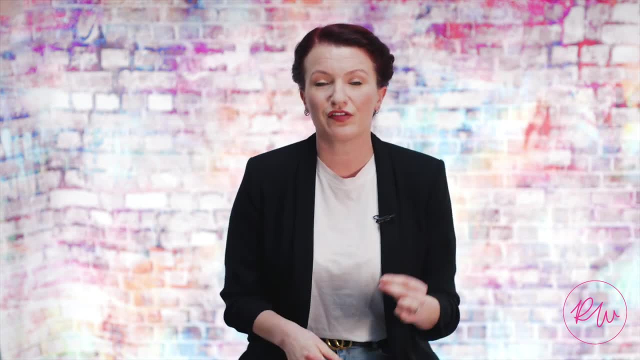 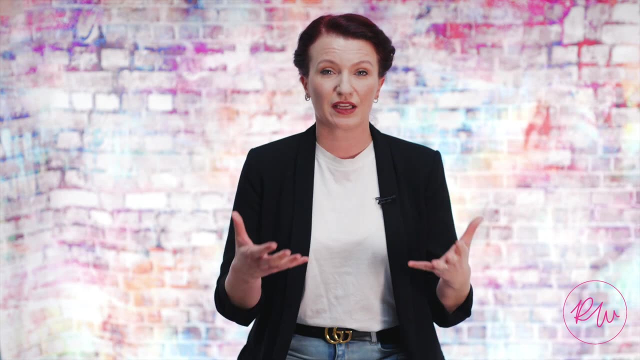 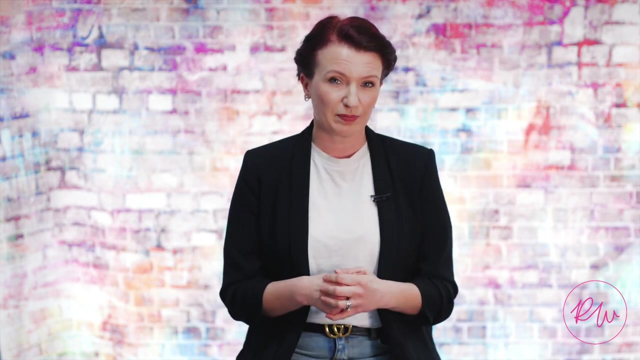 speaking online, remember to give yourself a moment to breathe before you start. Just giving yourself a moment, a couple of seconds, to take a good, deep breath before you start can make a huge difference to controlling your heartbeat if it's racing away. Also, when you are delivering your 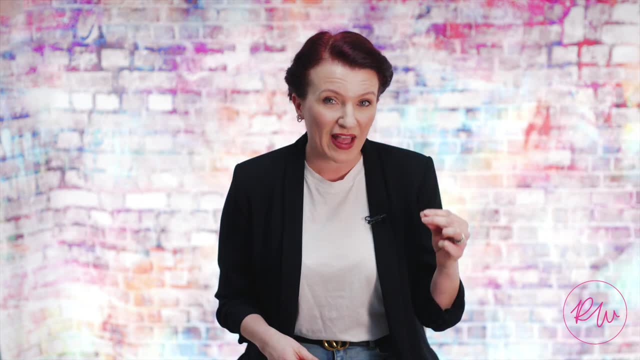 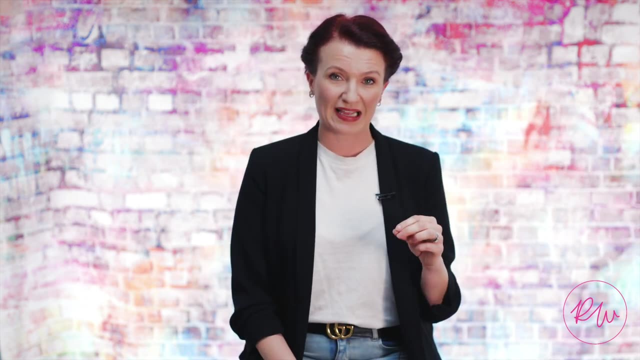 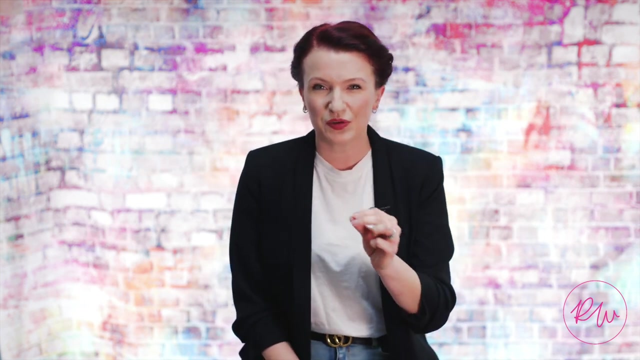 speech, your presentation. make sure you are aware at how fast you are speaking. Talk slightly slower than you would normally. If it feels a bit weird, then you're doing it right. You want to be talking slightly slower than you would say to a friend in the pub if you were in. 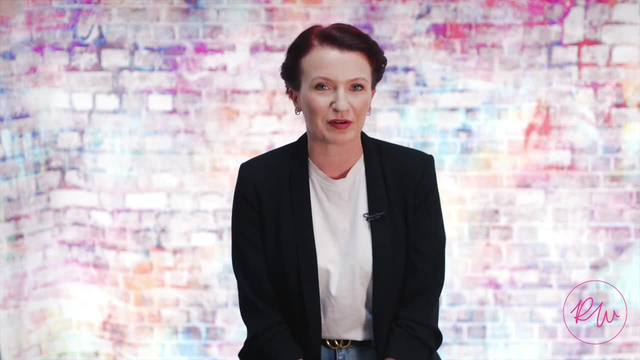 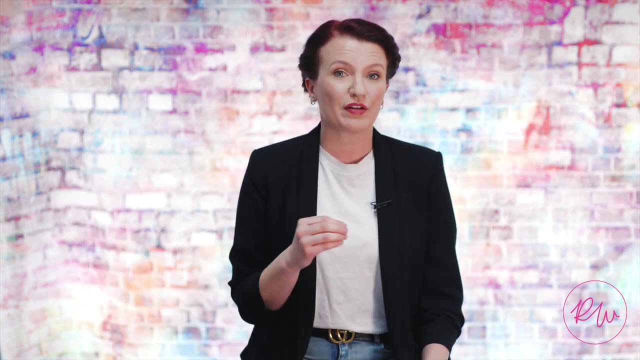 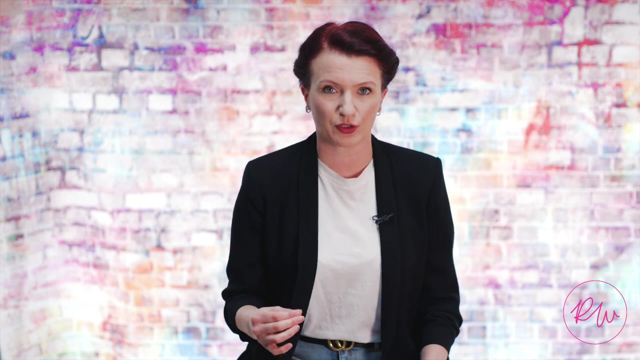 the UK, in the pub or bar, whatever. Tip number three is to use notes. If you are new to this, if you are nervous, notes can really help because it takes the pressure off feeling like you have to remember everything about your presentation. However, there is a good way and a bad way to 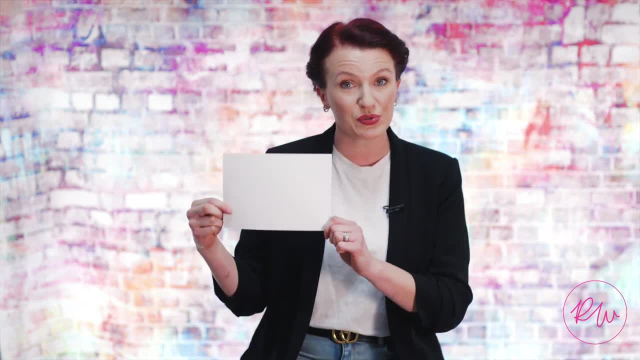 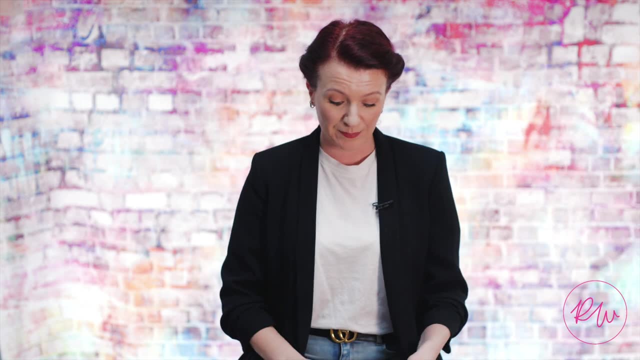 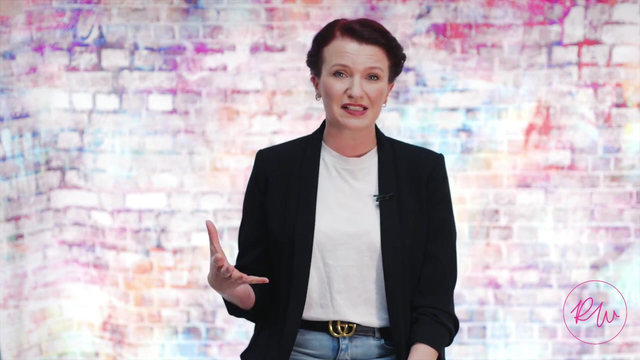 use notes. This is the good way. Use a cue card. Professionals use these all the time. just a piece of paper about this size. It doesn't matter if the audience can see it. If an audience sees a presenter using cue cards, it just says to them: this person is prepared, They've put effort into. 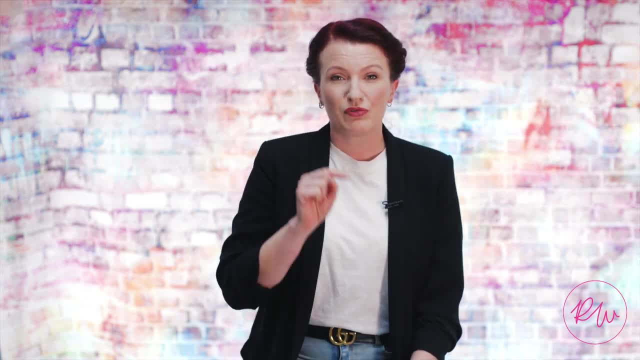 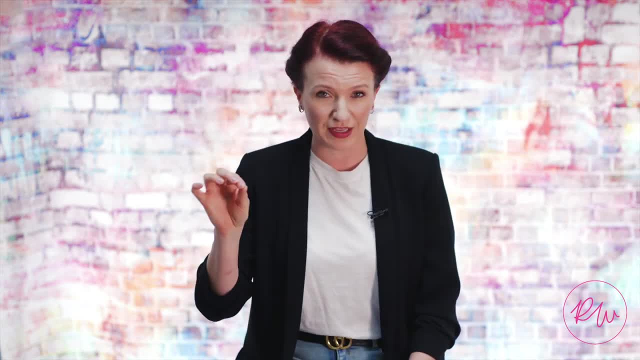 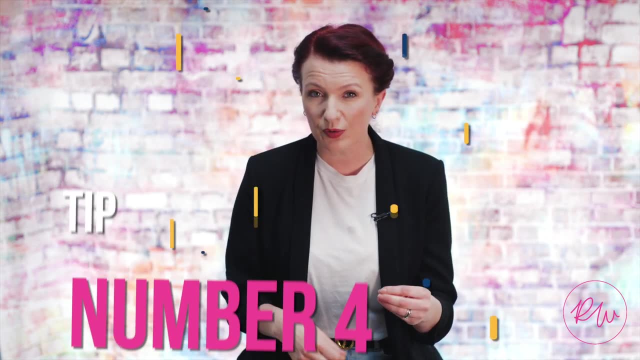 note them. If you are nervous, note them down. If you are nervous, note them down. There's a video here where I talk all about how to use cue cards. They're great. Use them. Tip number four: make sure that your slides, so your PowerPoint, for instance, relates to what you are saying. 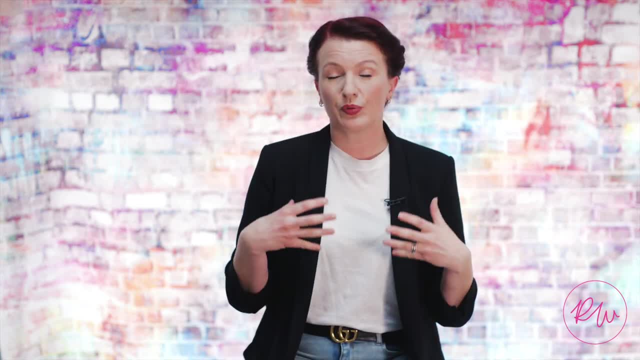 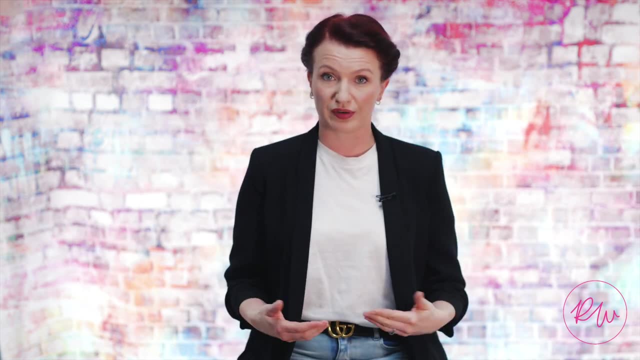 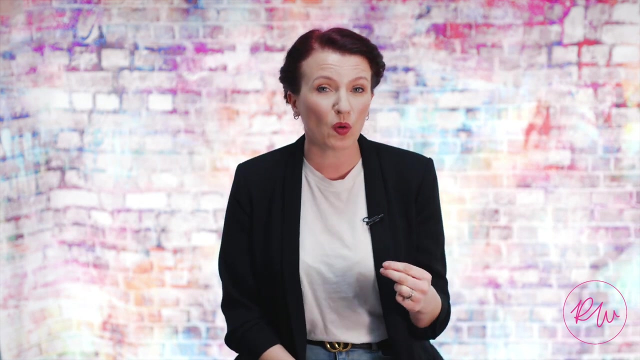 in your presentation. All too often, people who are new to public speaking or those who are nervous will rely on their slides to tell their story, to deliver their content. It's a bad way to go. your slides should only support what it is you are saying. I talk about this a. 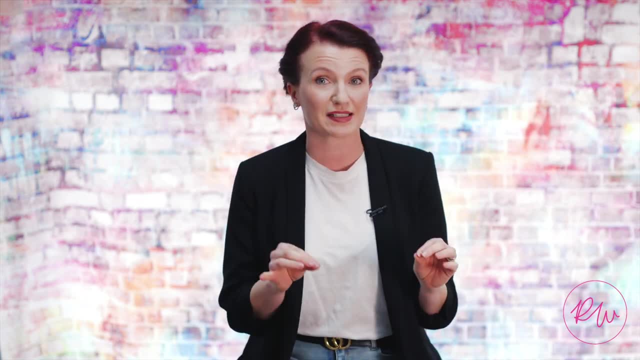 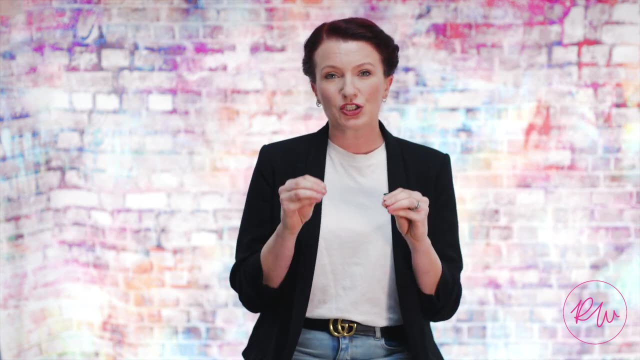 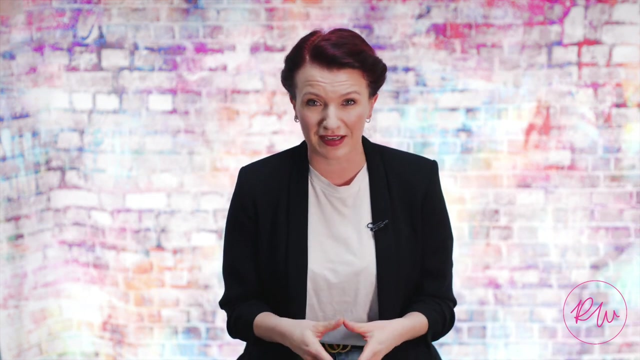 lot in my training course. if you're interested in that, which has a free PowerPoint template, then the details of that are in the description bar below. but make sure that what you're saying and what you're showing on screen are aligned together and don't fill your slides with endless text. tip number five: 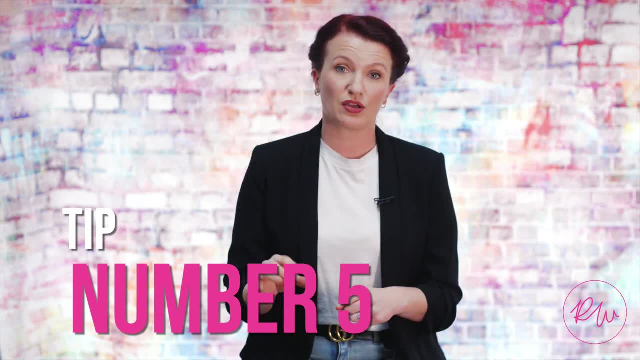 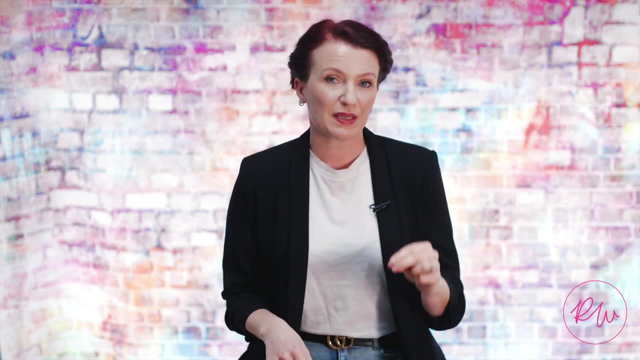 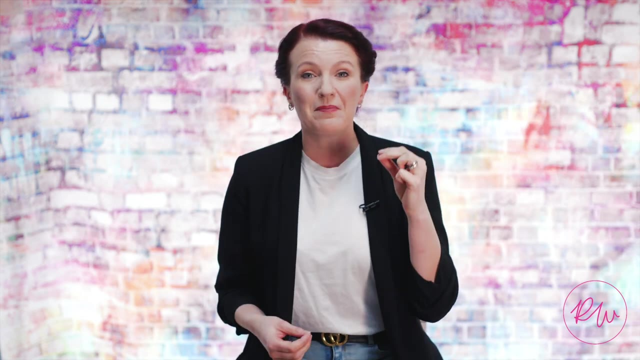 probably the one that will make the biggest difference to you, if you are new to public speaking and if you're nervous, is to practice out loud. most people practice their presentation in their head. they never say it out loud. there are many problems with this, but the main one is is that voice inside your head is 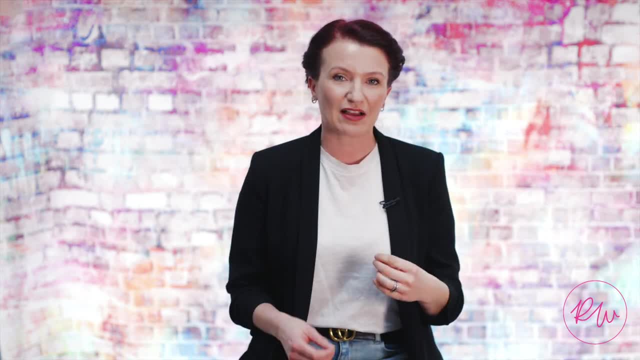 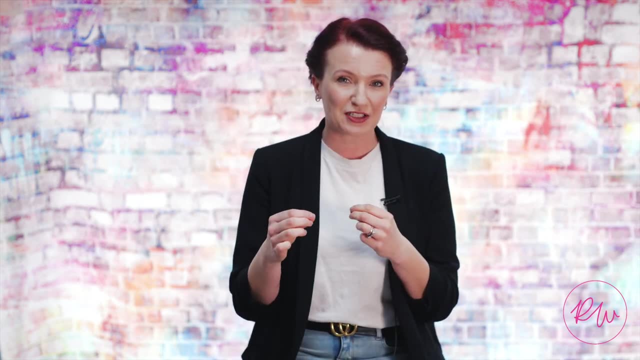 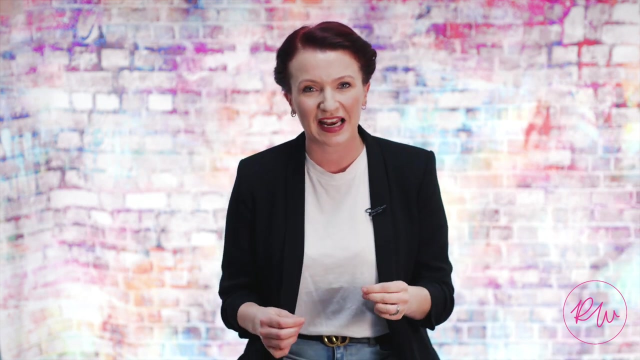 really good at reading what you have written down. when you say something out loud, obviously your brain and your voice is having to engage. that takes a millisecond longer than the voice inside your head takes to relay your content, and if you've never said it out loud, 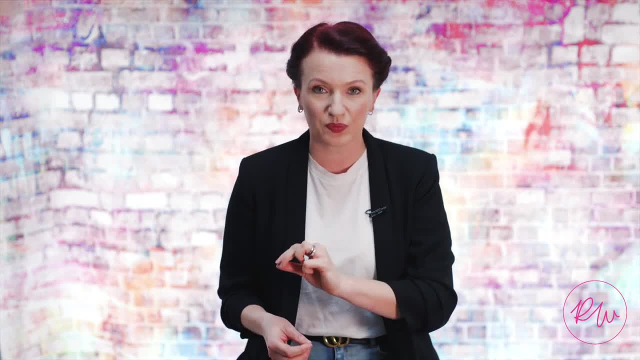 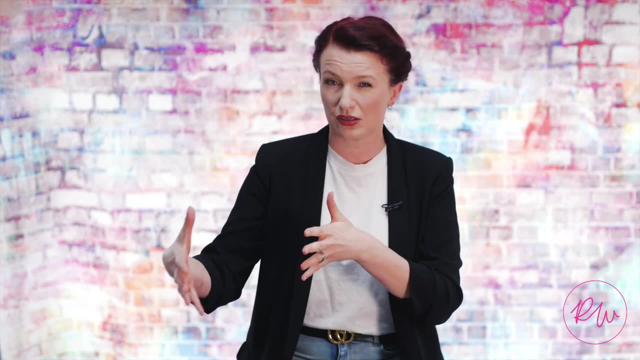 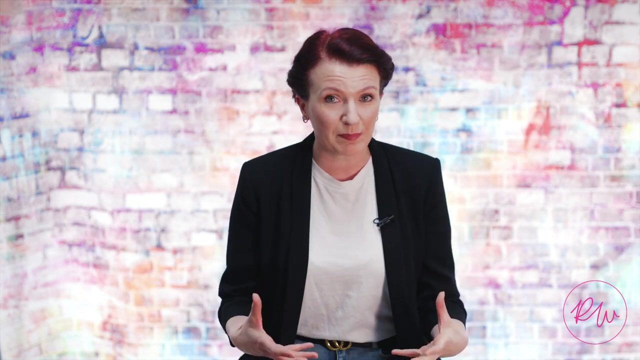 that is the point where you realize it doesn't work. sometimes, when you're saying content out loud, you realize that the structure of your presentation doesn't quite work, or you realize that the words that you plan to use are too difficult to say and you keep stumbling on them. so make. 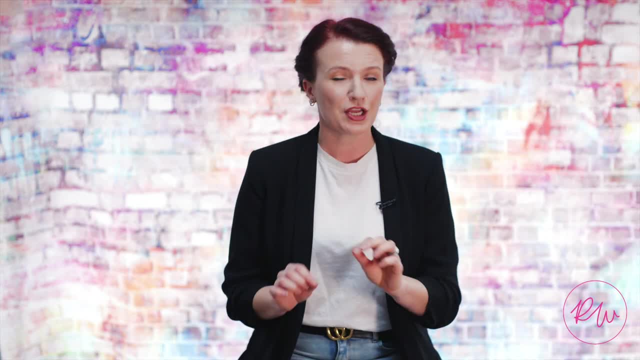 sure you do this well. so if you've had a few questions in the last couple of days, don't forget to put them in the comments section of the video. so I'll see you next time you say your presentation out loud, do not let the first time you say it be.